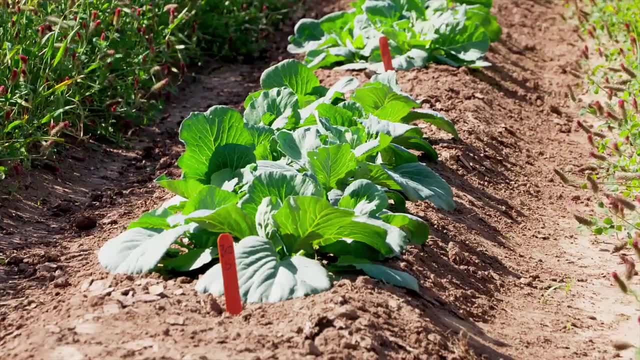 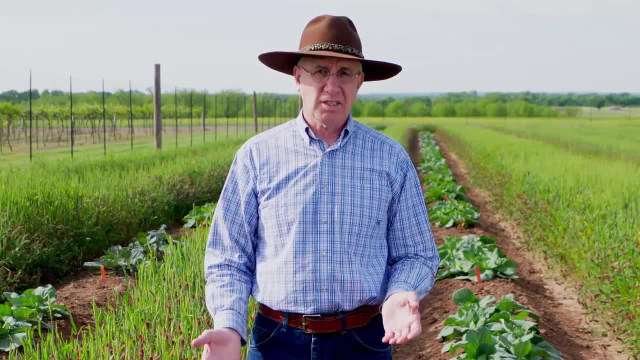 nitrogen per acre And that sounds like a lot and it is a lot, but this is a big, fast-growing crop, So one of the things that a farmer has to decide is how much fertilizer to add. So if you've taken a good soil sample and sent it in to have it analyzed, it will come back. 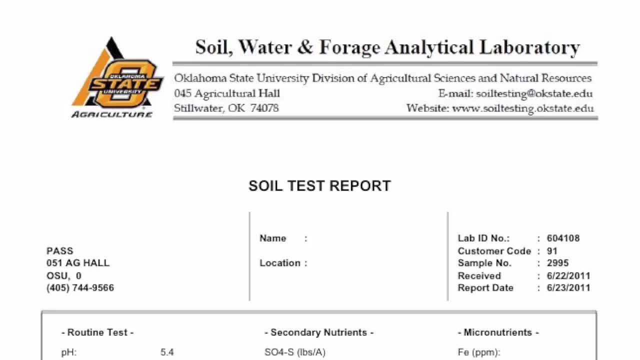 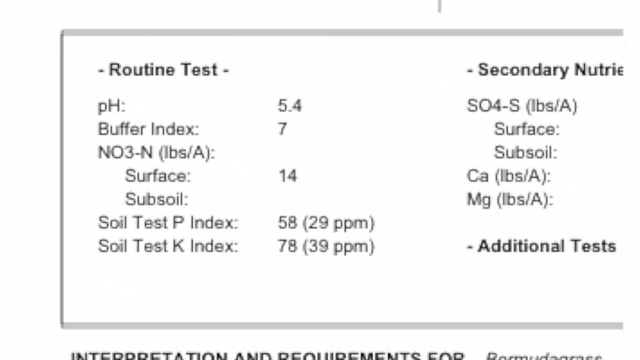 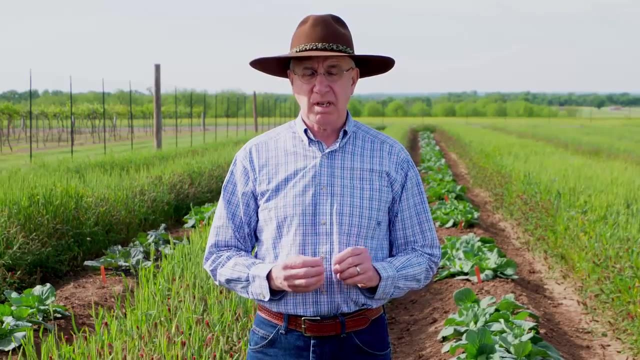 and it will give you recommendations for your particular crop. It will tell you how much nitrogen, phosphorus and potassium to add If your soil pH is too low or too high. it will tell you what to do to help adjust that soil pH, And pH is a critical part of soil. 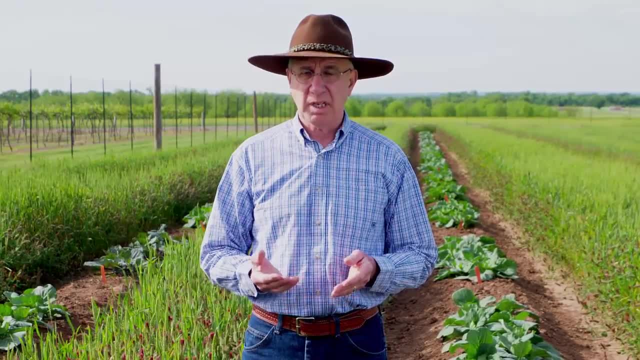 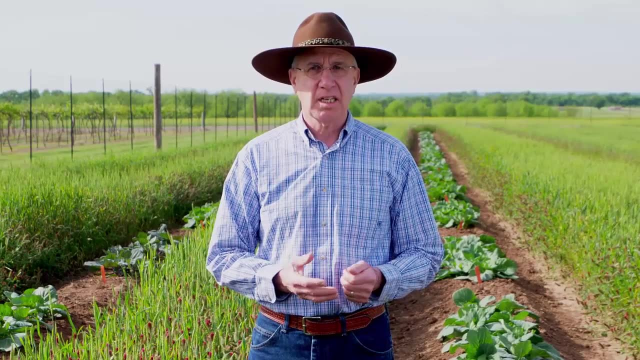 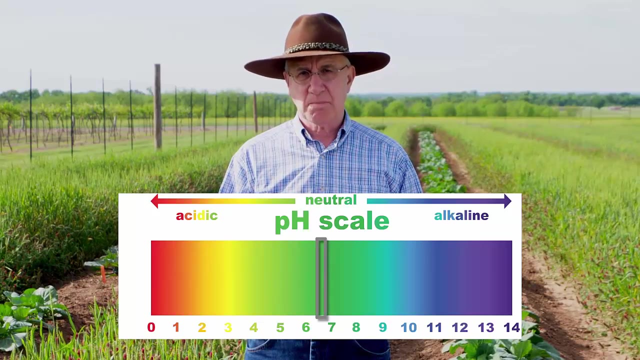 fertility, because soil pH affects the release or the availability of all the nutrients for the crop. Where all vegetable crops want to be is slightly acidic. So on a pH scale which runs from 0 to 14, we'd like to be somewhere between 6.5 to 6.8.. You know, if you're in the low 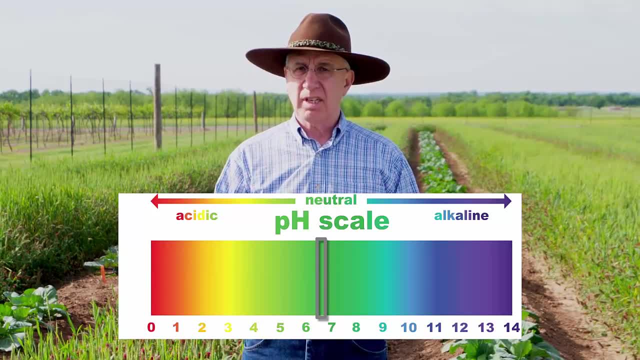 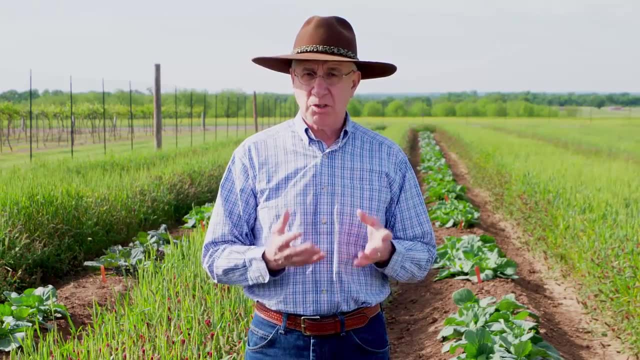 sixes, you're 6.2,. 6.1,, that's okay. If you're in the high sixes, or even 7,, you're all right, But the ideal spot is that 6.8.. That will make the most nutrients available to the crop. 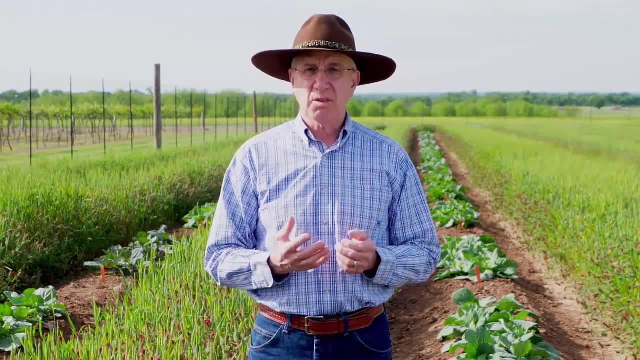 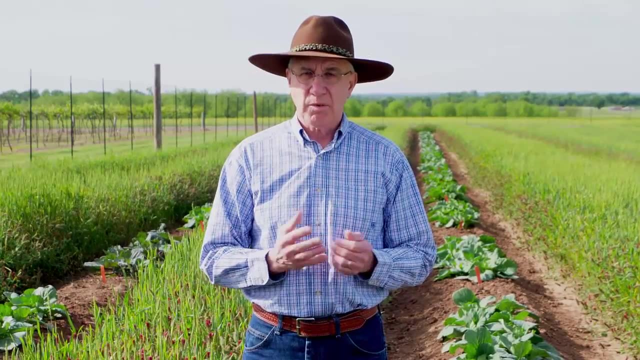 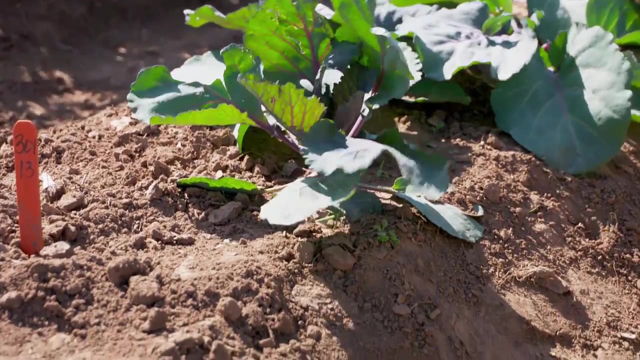 and it will grow the best at that pH. The other thing that goes on with soil is it basically stores nutrients and it stores water for the crop to use. It also provides the ability for the crop to root down and to be anchored in the soil. 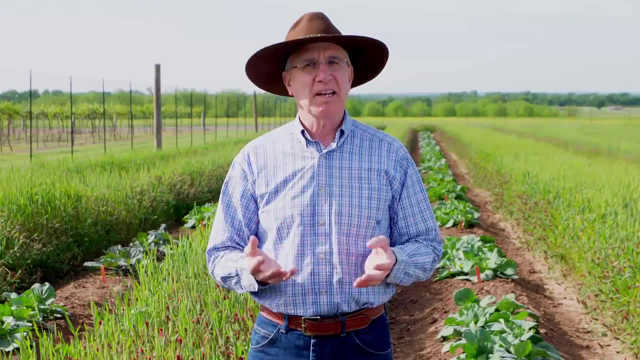 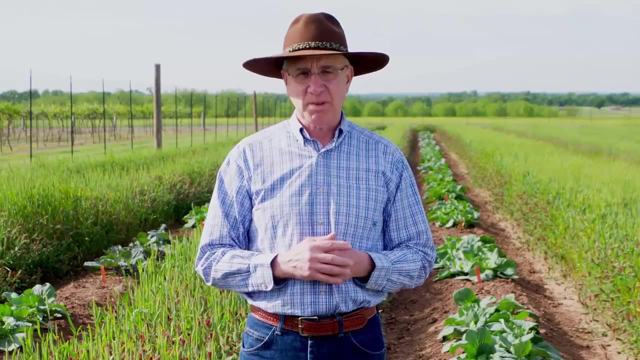 Now, if you live someplace that the wind never blows, you might not understand that, But in Oklahoma, where we get 60, 70 mile an hour winds, anchorage is important. Trust me, it's very important. The other thing that: 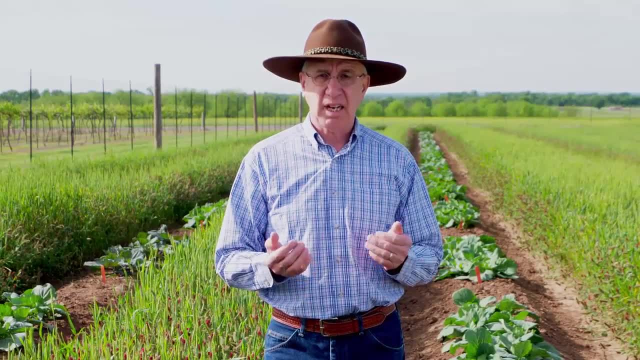 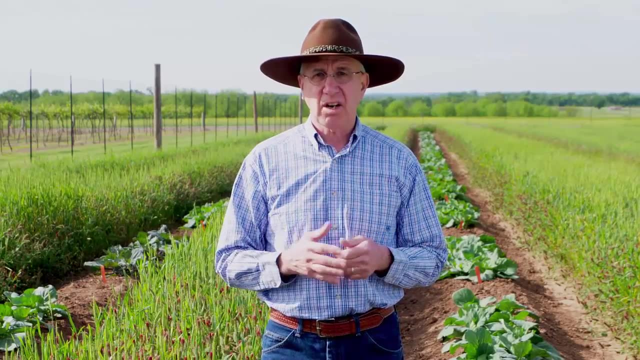 soil fertility, managing it properly does is that it allows you not to waste money or nutrients. You know, if you're just kind of taking a shot in the dark and you're putting out fertilizer and you think, well, that'll be good and it might work, But a lot of your money and 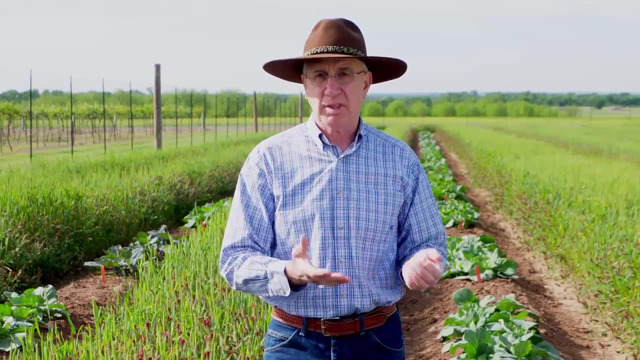 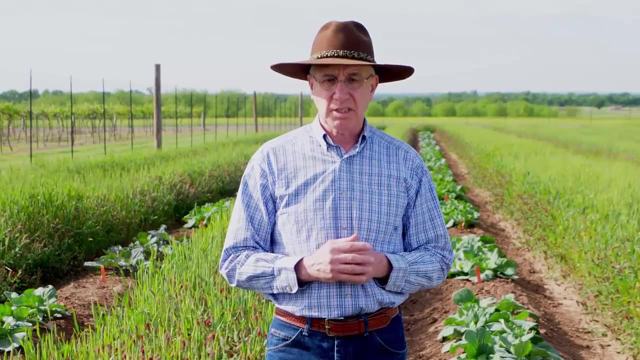 nutrients may be wasted because they're excess from what the crop can actually use. So it's important to get that soil test result back and then to follow those recommendations. Last but certainly not least, we really want to talk about the importance of taking care.